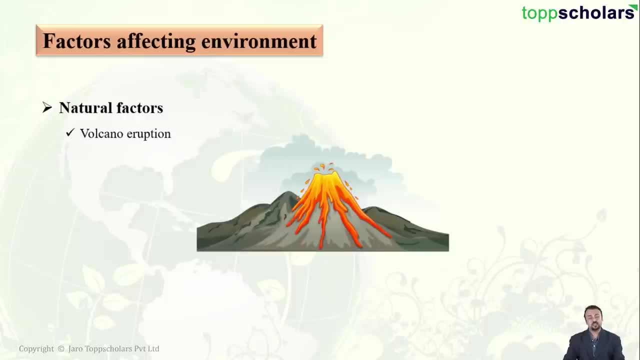 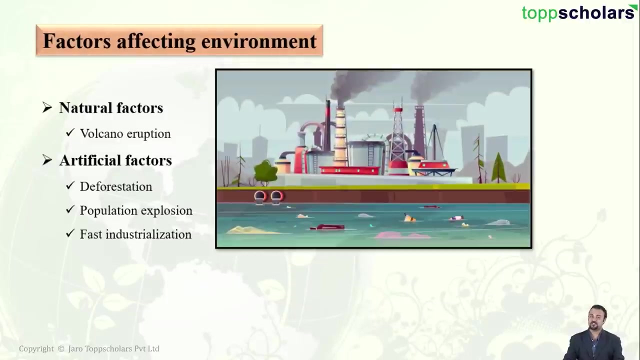 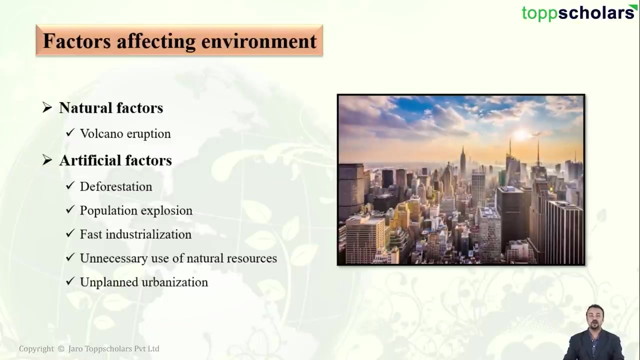 cause too much damage to the environment. What actually is causing the damage to the environment are the artificial factors, or we can even call them the man-made or anthropogenic factors, such as deforestation, population explosion, fast industrialization, unnecessary use of natural resources and also students, unplanned and over urbanization, Students- what is environmental? 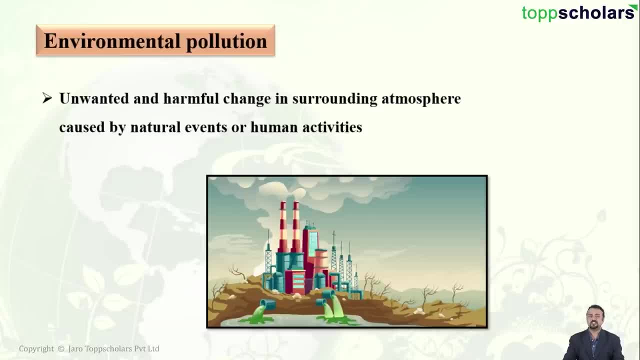 pollution: Unwanted and harmful change in the surrounding atmosphere which is caused by the pollution of the environment. What is environmental pollution? Unwanted and harmful change in the surrounding atmosphere which is caused by the pollution of the environment. What is environmental pollution? Unwanted and harmful change in the surrounding atmosphere which is caused by. 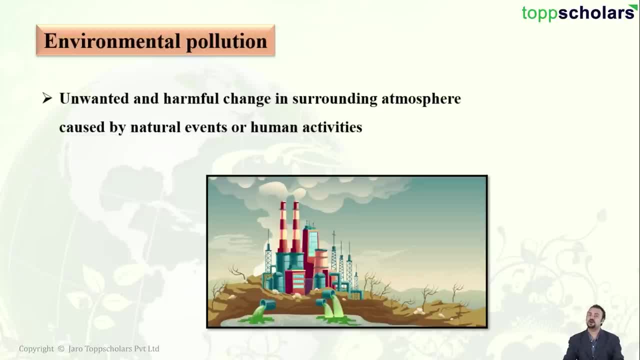 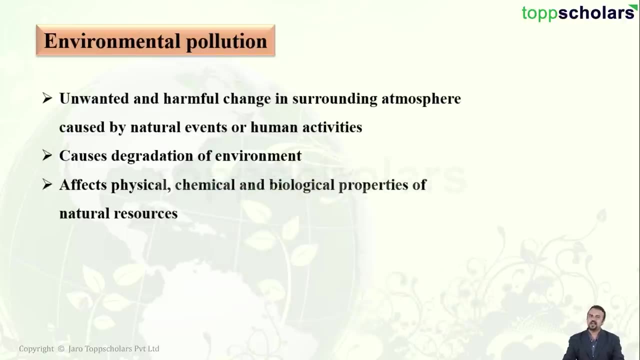 natural or even human activities is called as pollution. Now, this unwanted or harmful change can cause degradation of the environment, And when I say cause, it has already caused the degradation of our environment and it can affect the physical, chemical, as well as the biological. 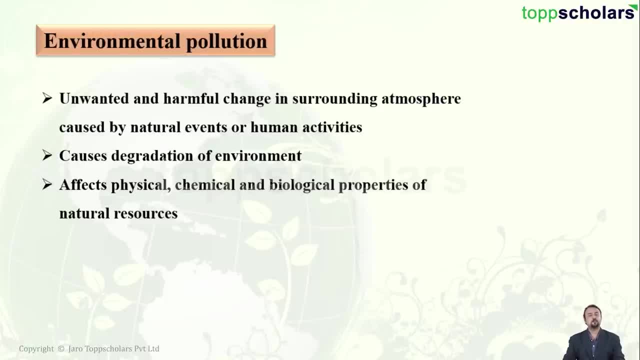 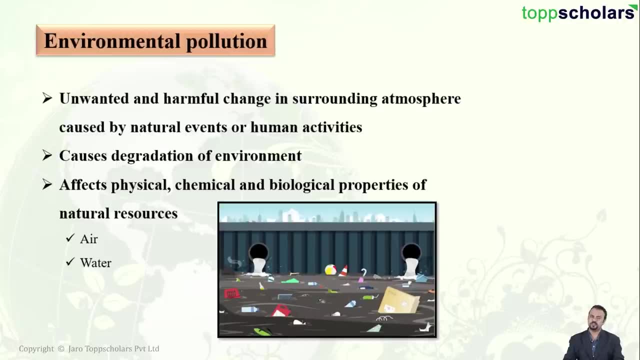 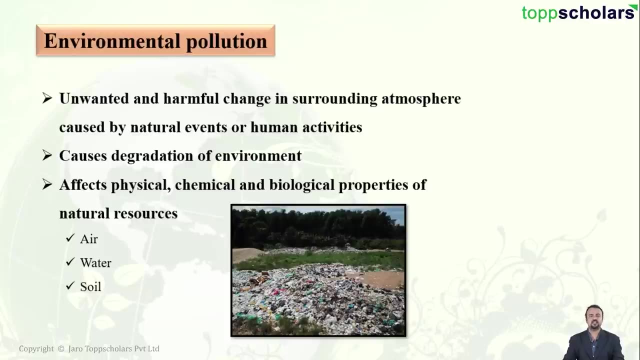 properties of various natural resources. Pollution, students, mainly is of three types. The first one is air pollution. The next one is water pollution. The second one is water pollution. The third one is soil pollution. These are the three major types of pollution seen in the environment. Moving on, 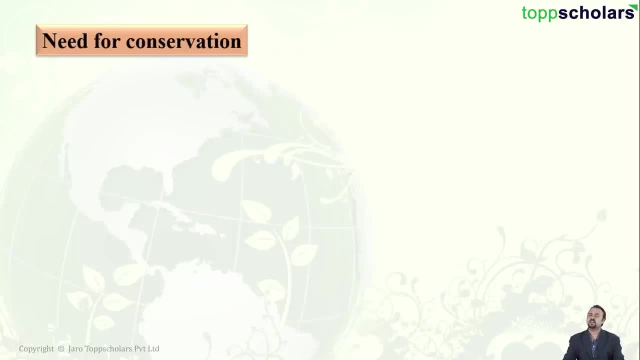 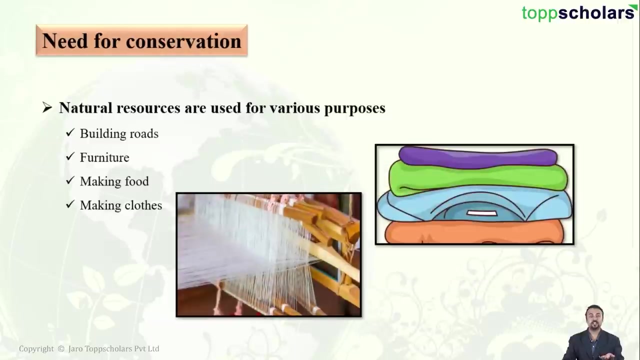 students. now let us understand what is the need or the requirement of conservation. Students, natural resources all around us are used for various purposes. For example, they are used for building roads, They are used for furniture, making food, as well as making clothes. Now, I don't have. 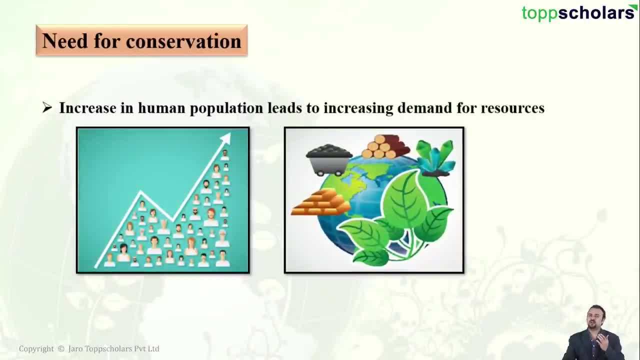 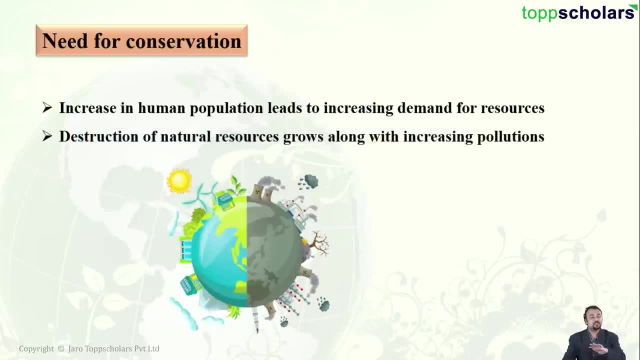 that when the population goes on increasing, there is obviously going to be increase in the demand for natural resources. Now, what this will do? it will completely destroy the ecological balance, as well as completely deplete the natural resources. Moving on, students, it is very, very. 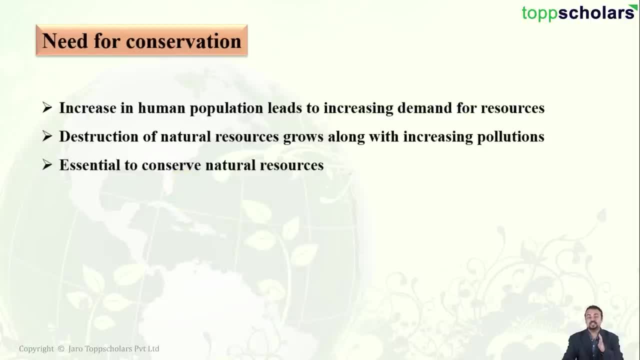 important for us to conserve these natural resources because it will maintain the ecological balance and also we need to think about the future generations. For example, if we have a wild animal, for example, even some wildlife animals like a tiger can be considered as a natural. 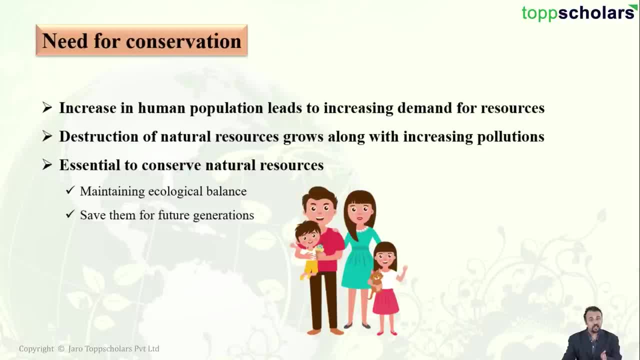 resource, and if we don't conserve them today, then the future generations will be only able to see pictures or images of the tiger, So therefore we need to save them for our future generation. To learn more about this topic, download Top Scholars app.